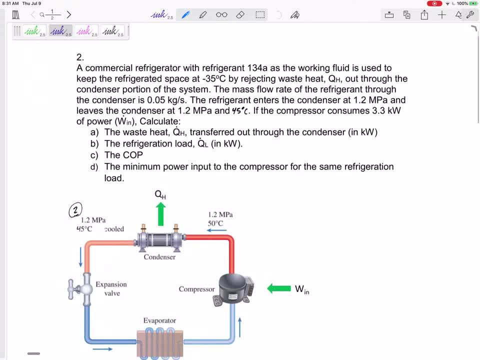 Okay. so these refrigerator problems are easy, too easy. How might they get harder? Well, here we go. It gets harder when they don't just give us the Q H or the Q L or the W on a silver platter. Okay, so now we might kind of need to look inside the refrigerator at all. 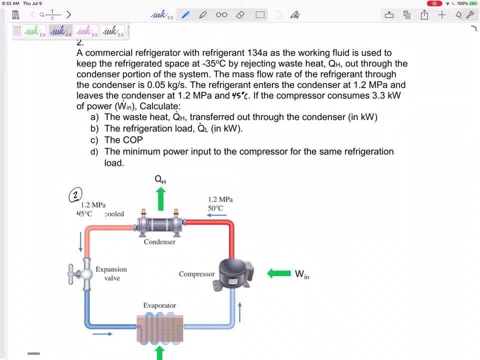 the different components of the refrigerator and really look at the working fluid. and hey, what are the properties of the working fluid before the condenser? What are the properties of the working fluid after the condenser? And if we know the properties before and the properties 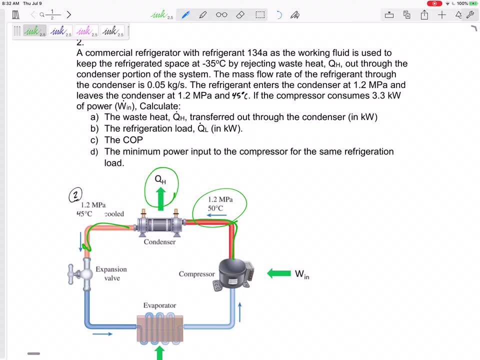 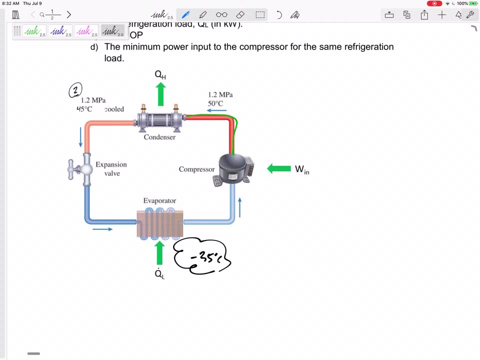 after maybe we can find this Q H that's going to come out of there. So that's what we're going to do. So here we go. We've got a refrigerator using refrigerant. It keeps the refrigerator space at negative 35 degrees. That's talking about this. outside this space, negative 35 degrees C. 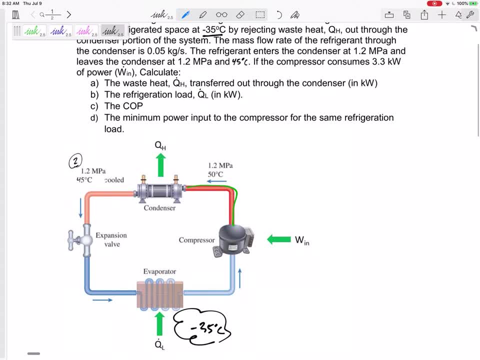 That is not talking about the refrigerant Refrigerant inside of here, right, It's not talking about the working fluid. That's just talking about the refrigerated space, And I think we're going to use this later, not today, But I 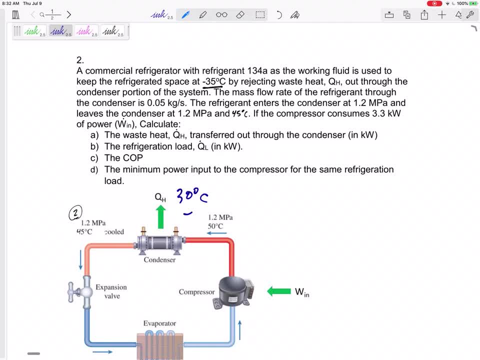 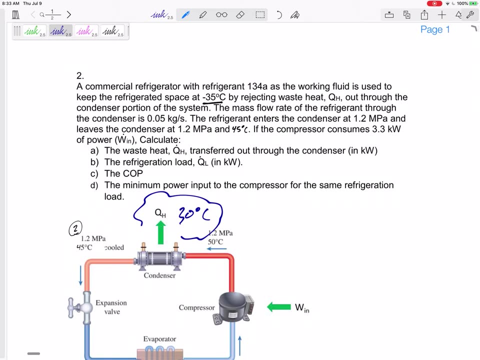 think if the room, if it's spitting this Q H out into the room and the room's at 30 degrees C, we might use those later. We're not going to use those today, But anyway, don't get the. 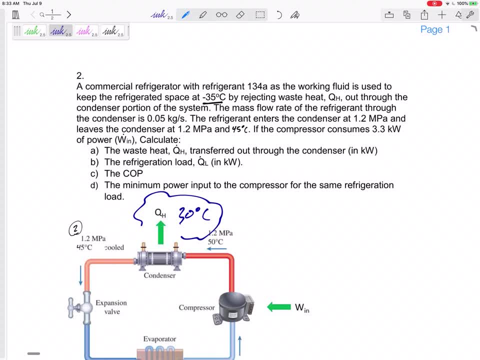 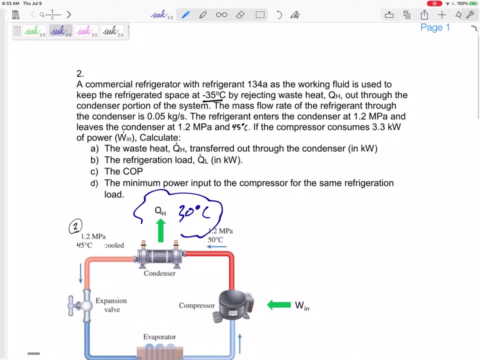 the temperatures of the air and the working space and the area behind the refrigerator. Don't get confused with the temperatures of the that's that's inside of the refrigerant going through these different devices. Okay, So it's using refrigerant 134A. It rejects Q H out through. 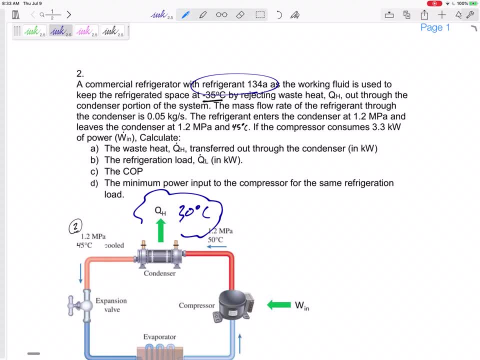 the condenser portion of the system. The mass flow rate of the refrigerant through the condenser is M dot. right, That's M dot is 0.05 kilograms per second. The refrigerant enters the condenser at a pressure of 1.2 MPA and a temperature. 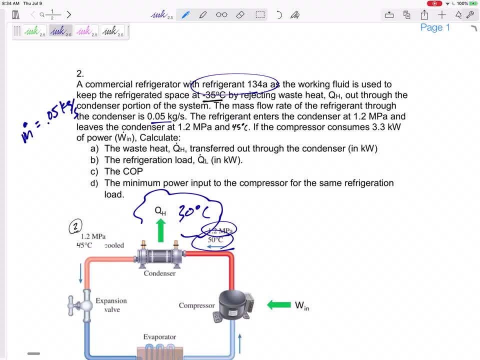 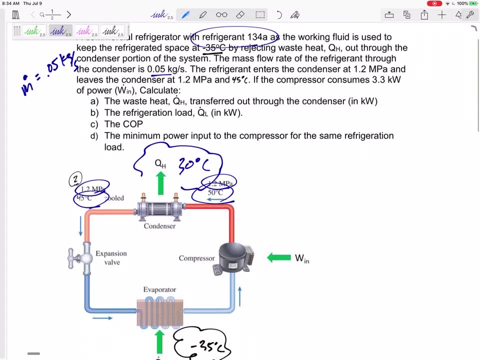 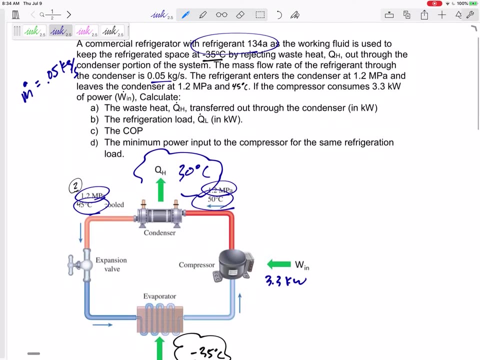 of 50 degrees C, It leaves the condenser at 1.2 and 45 degrees C. If the compressor consumes 3.3 kilowatts of power, so 3.3 kilowatts of power in. then calculate all this, the Q, H, Q, L, the COP, And we're going to do. 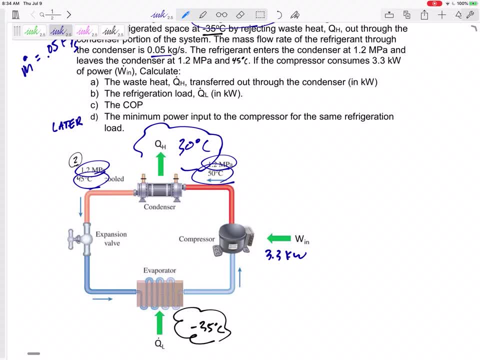 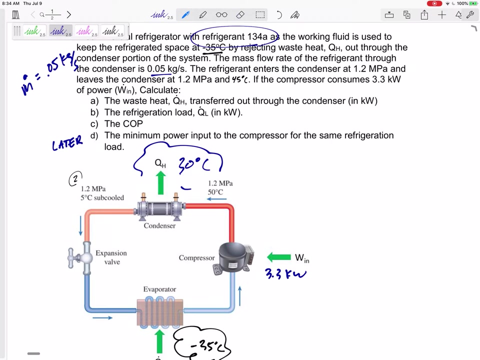 part D later, because we haven't talked about that- The minimum power that would be if this was an ideal compressor, if this was a Carnot or reversible- we'll talk about that later on. Okay, So here we go. Do you see that if we know the properties of the refrigerant as it's going into the condenser and as it's going out of the condenser, 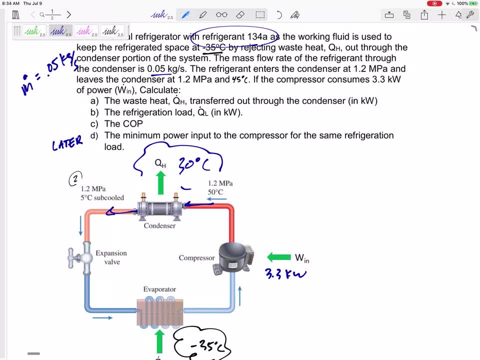 we can use conservation of energy to figure out. we can use conservation of energy to find Q right. Q plus W equals: well, this is a steady flow. This is a steady flow device. equals M, dot And really H is the only thing. that's, you know, not negligible, right, Remember. go back to steady flow devices. Remember sometimes you have kinetic energy when we're really worried about velocities, but we're not worried about velocity of the refrigerant, Sometimes potential energies. if we have large changes in height, those are going to be negligible. So it's our 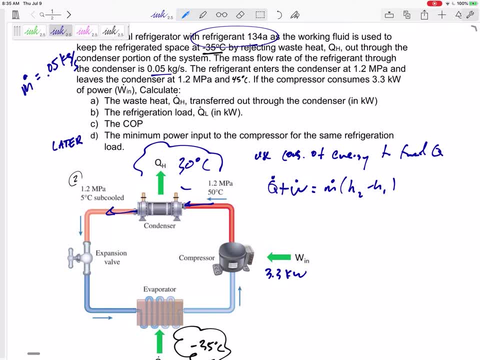 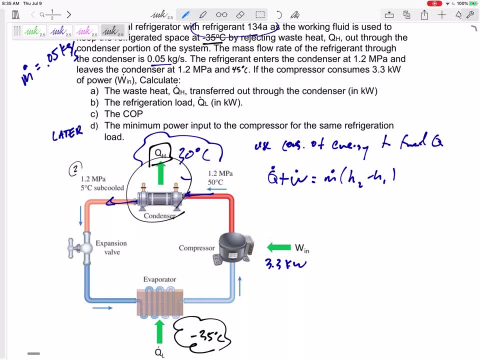 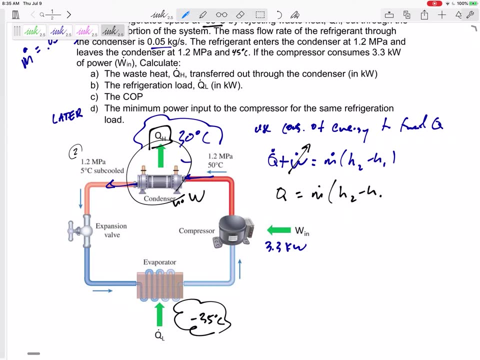 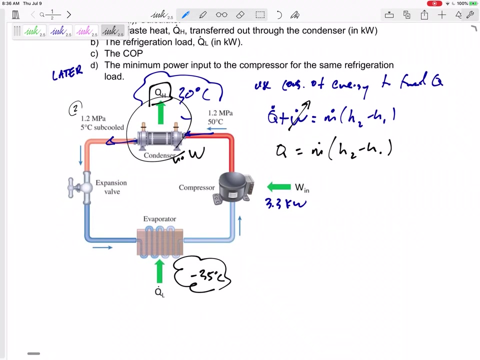 conservation of energy is really just boils down to Q plus W equals M delta H. Right here at the condenser there is only Q, There's no W, And so it's really M dot change in enthalpy, M dot change in enthalpy. All right, So that is how these get these refrigerator problems. get a little bit hard, It's not that bad. 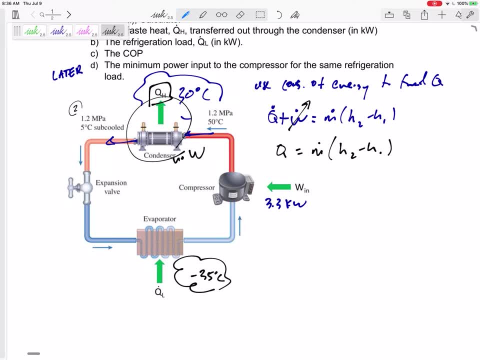 It's actually a little bit of a twist in here. Instead of giving us the Q, they tell us the properties before and after we get the delta H times M dot. That's the Q Sometimes. sometimes they'll do that over here. So over here the conservation of energy would be: W equals M dot delta H. Maybe we shouldn't label these two and one, but the change in delta H, Or maybe they do it down here: Q plus M dot. 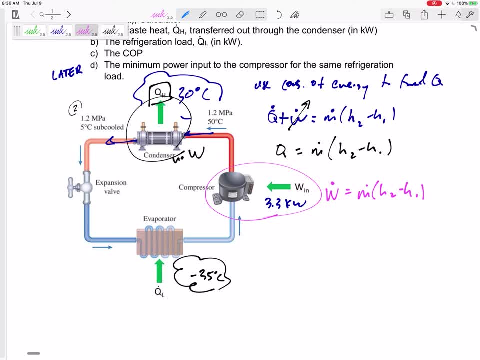 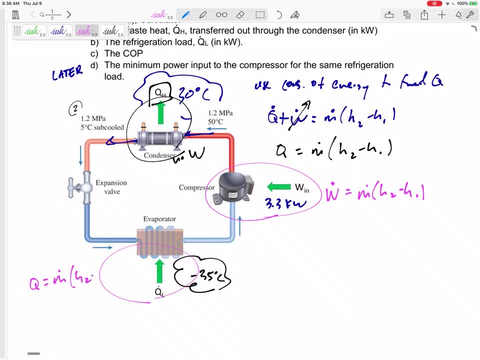 Okay, Okay, Okay, Okay, m dot right, so. so sometimes they don't give us the q or the w, they give us the properties of the fluids right before and after it goes into whatever device that we're they're looking at. if we know the properties before and after, we can find the h's. if we know the h's, we can 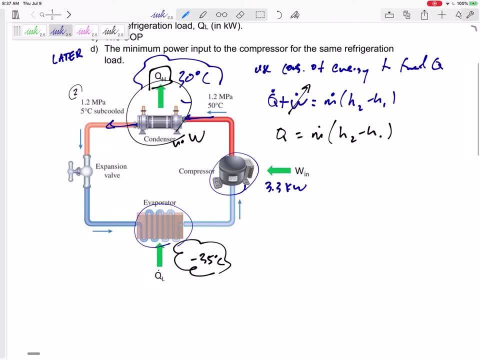 m dot. delta h equals q. all right, so let's, let's look at this before and after. so let's think about this like state one: if the pressure is 1.2 mpa, if the temperature is 50 degrees c. so you thought we were done with property tables. you thought we were done with all that? no, we're. 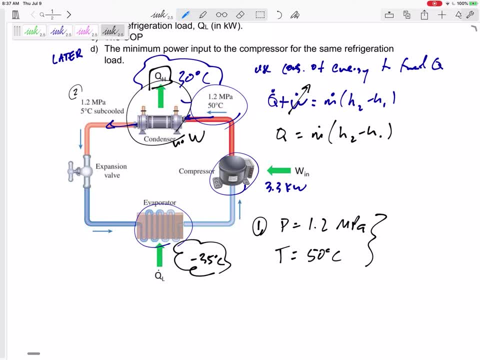 still using that. so from that you know, you go see: is it saturated, is it superheated, is it sub cooled? hopefully by now you can find the enthalpy. look at through the tables. 278.28 kilojoules per kilogram. is is what i've got. uh, but what if the pressure is 1.2? 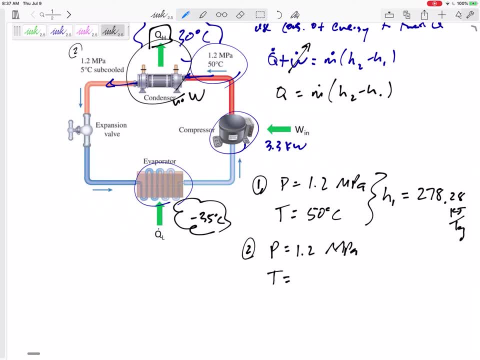 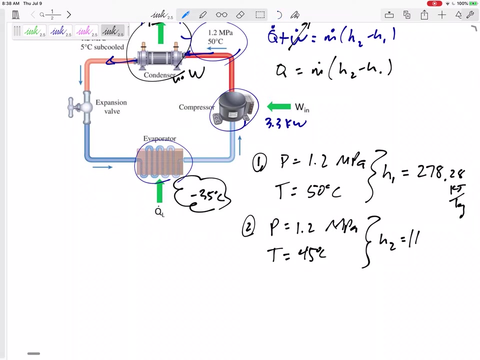 and the temperature is 45 degrees c. look through there, i don't have this written down. did it become a sub cooled liquid or is it still superheated just at a lot, at a different um, um, h, um, this big change in h, i think? i think it may have been, uh, sub cooled now, uh, but, but look at that, okay, so i'm not going. 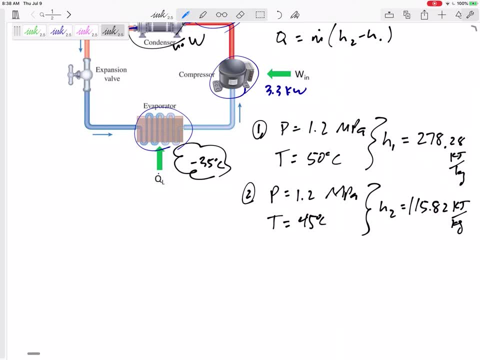 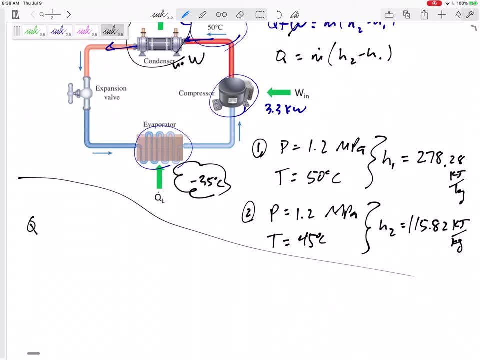 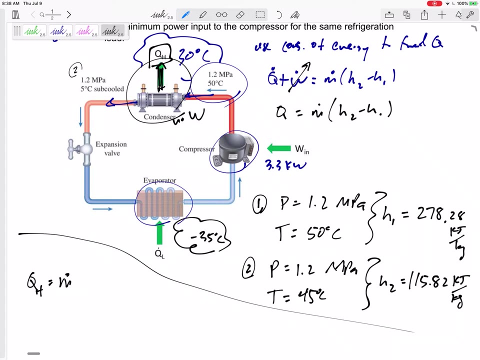 back over that. you should be able to find those properties, find the h given the properties right before and after. so the q now is this q h or q l? this is q h because we're looking at the condenser here. q h is m dot. change in h. q h would be. 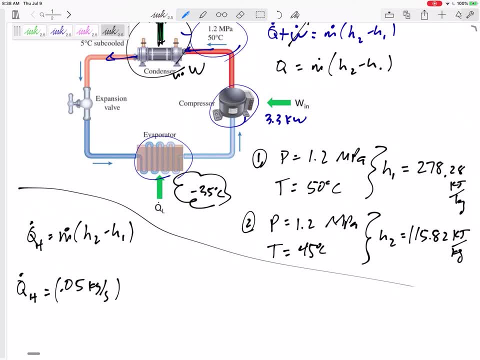 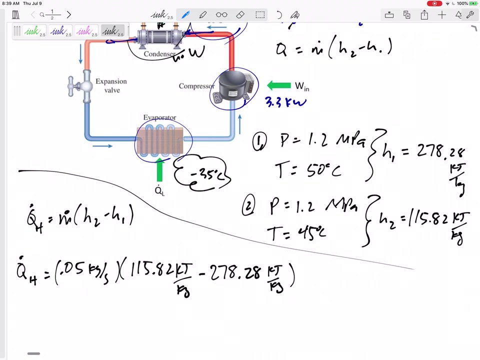 0.05 kilograms per second. let me think about units here. h2 was 115.82 kilojoules per kilogram, minus minus the initial 278.28 kilojoules per kilogram. all right, so kilograms can't solve kilojoules per second. kilojoules per second is a kilogram. 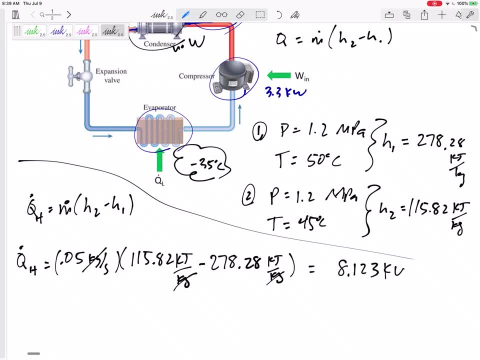 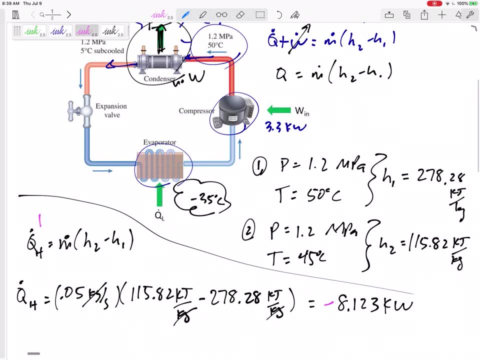 kilowatts, so this is going to be 8.123 kilowatts. now the math told me this was negative. what does that negative mean? that negative means it's going out of the refrigerant right, because this is for refrigerant right. that's the h of the refrigerant. the q of the q of the refrigerant is negative. yeah. 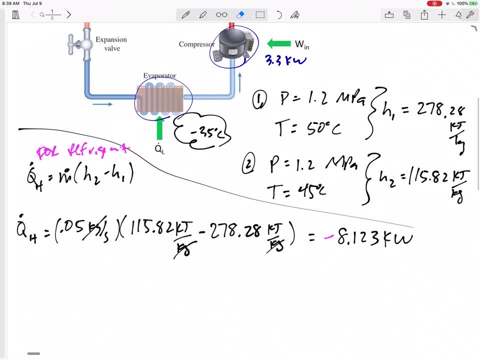 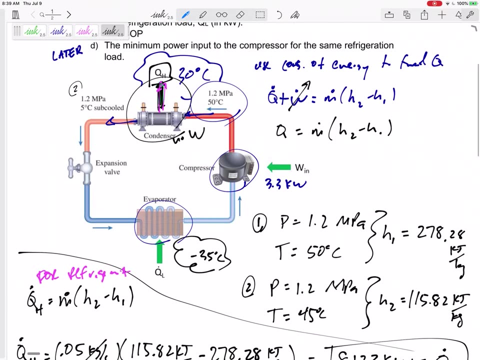 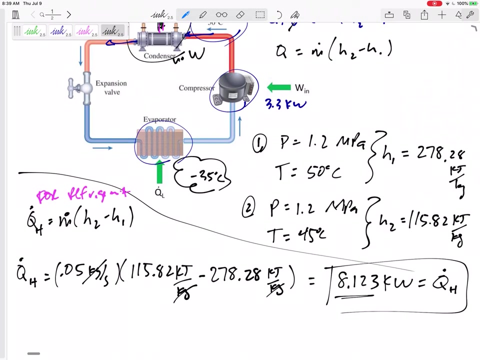 it's. it's going out of the refrigerant, so anyway. so the q h is. we already knew it was going out. the waste heat transferred out is 8.123 kilowatts. all right, that's the hard part. now let's go back to all those cop. is cl over w or w? is q h minus q l? let's go back to those easier equations. 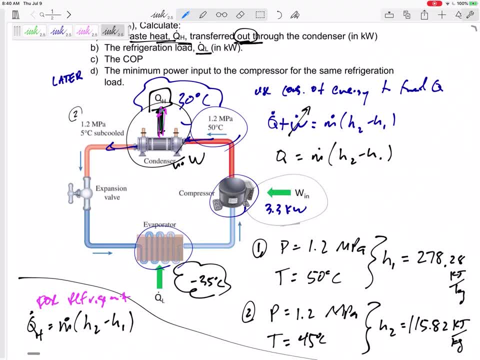 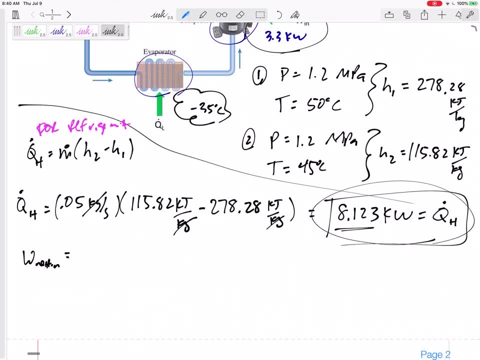 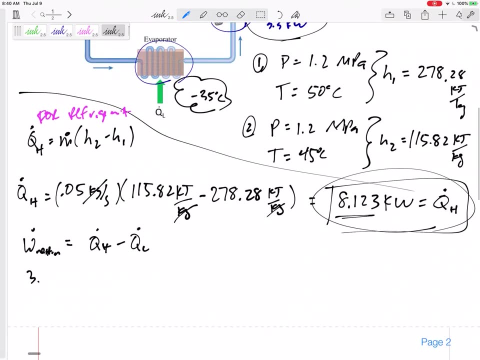 to find the q l. all right, i know the wn, i know the q h. how can i find the q l? w is q h minus q l, and i know this is three point. where were we sorry? 3.3, 8.123, q l is 4.823.